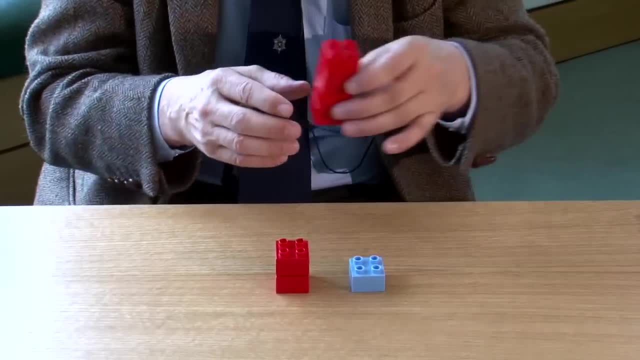 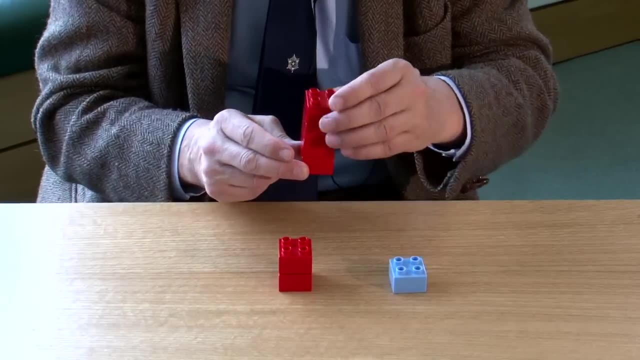 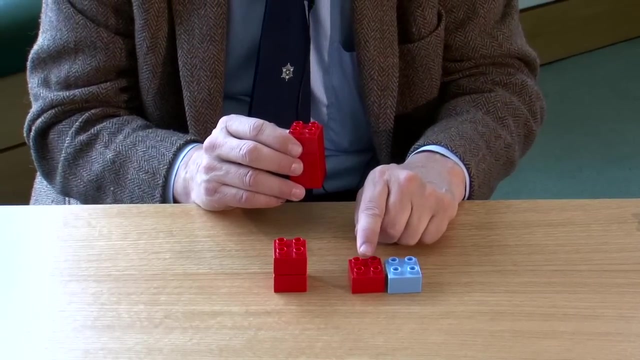 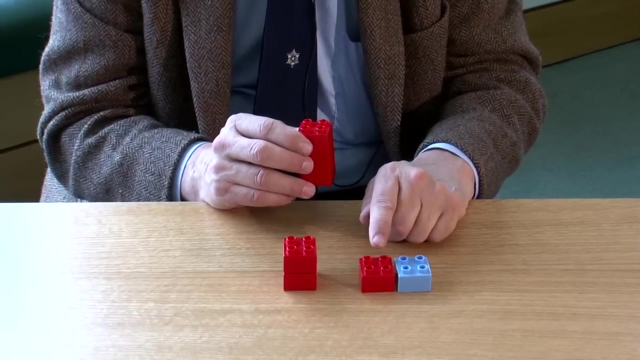 What has happened during my lifetime is that we became 4 billion more in the world and the richest became even more rich. Where have these extra ended up With? 1 billion is actually where the West used to be, like successful China, Brazil, Turkey. They acquired the Volvo company, so we know that they are just back of us. 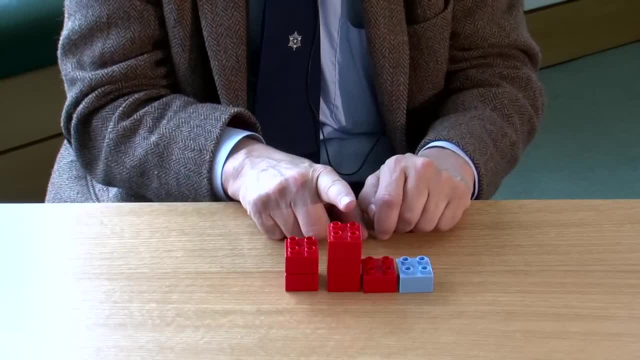 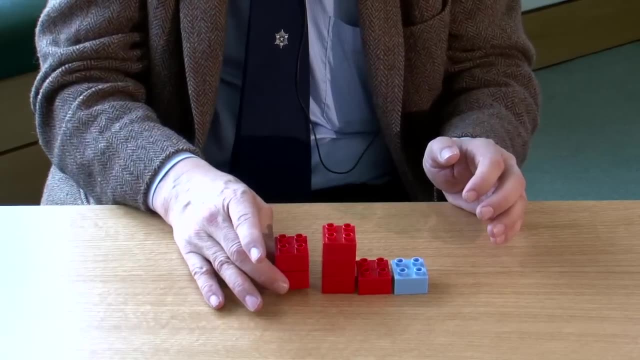 And 3 billions are here. They have a relatively decent life. They are 2 billion. Children go to school, but they live under a modest economic situation. 2 billion are almost as poor today- 1 or 2 billion- as it was before. 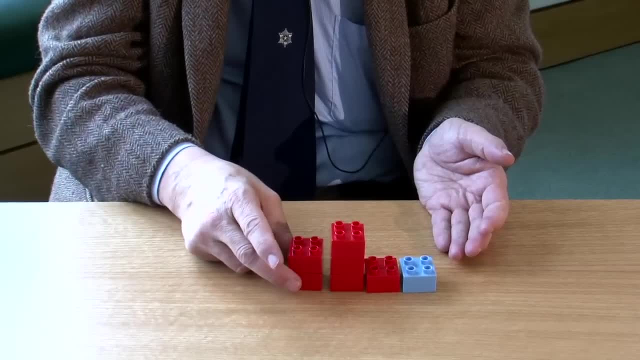 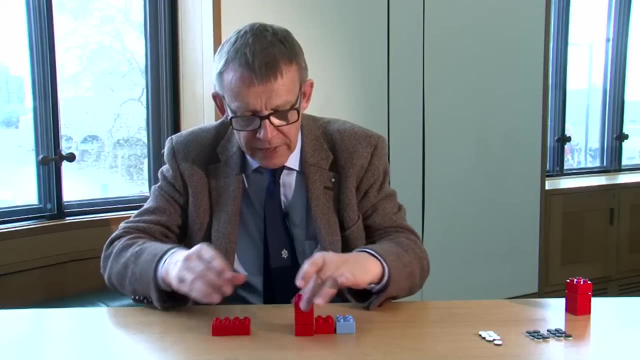 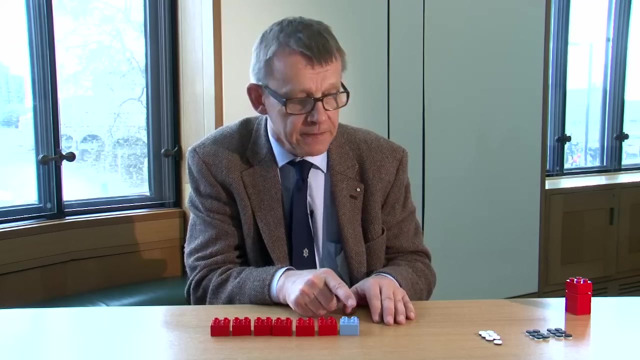 The poor are a smaller proportion of the world population, but their numbers are almost the same. Now, if I would place them in a sequence, the very poorest, 2 billion. these billions, imagine the 7 billion people in the world, from the poorest to the richest. 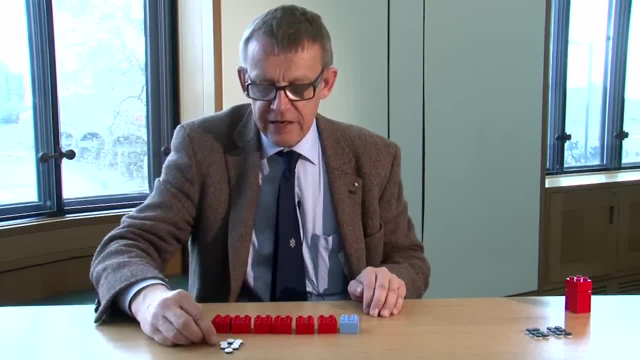 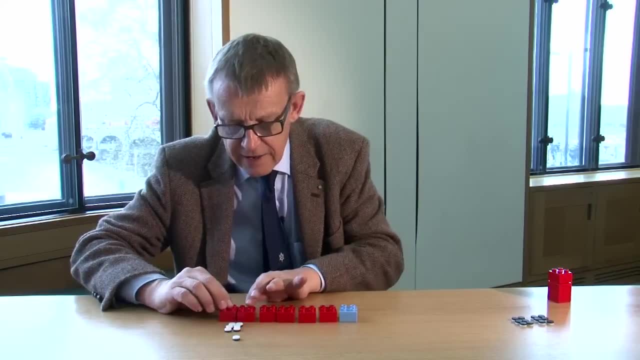 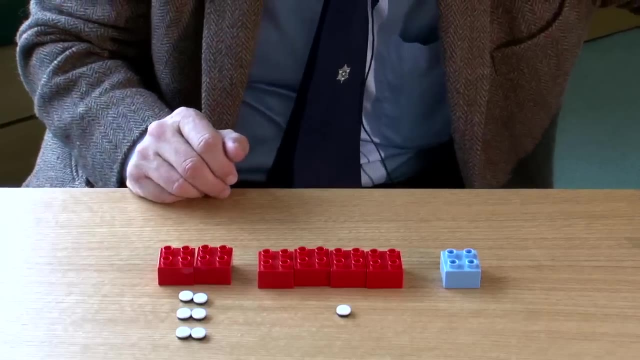 And we have 7 million children who die every year. 7 billion people, 7 million children die. 6 of these die in the poorest. 2 billion 1 die here in the middle and here almost no one. Where are then the fossil fuel emission? if this is all the carbon dioxide emission in the world? 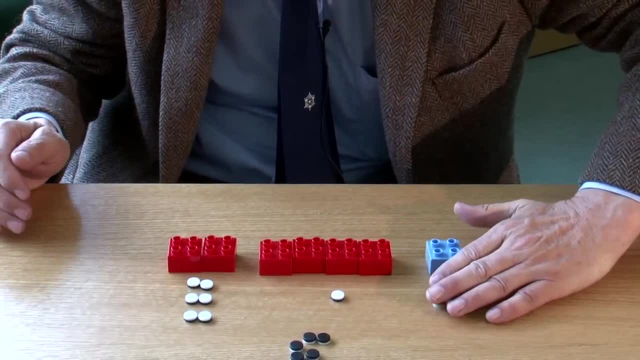 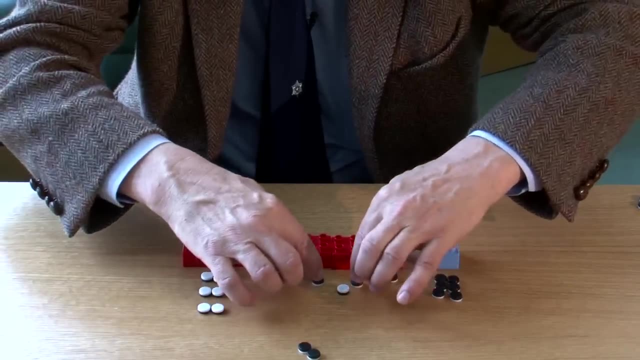 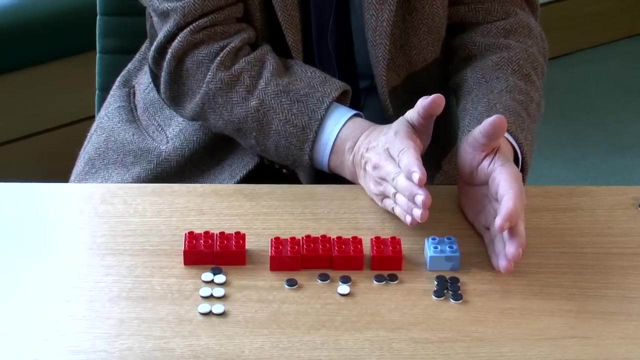 Almost half of it has been here now the last decade with the richest people, With the richest 1 billion. There are 2 units here. there is 1 unit each here and only 1 unit for these 2. It's very unevenly distributed into this direction. 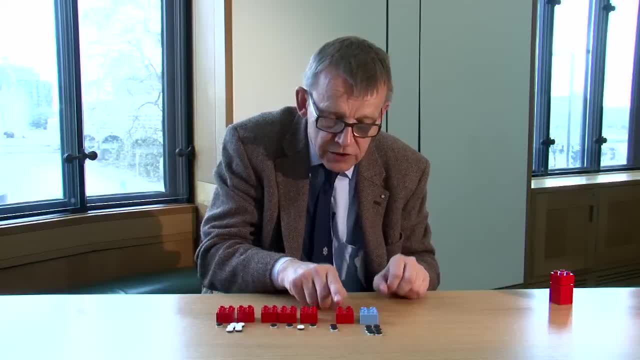 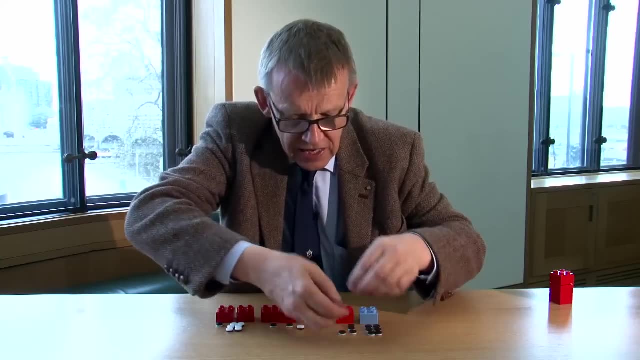 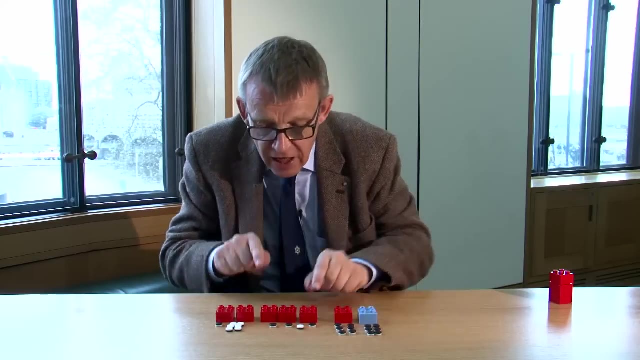 They really emit a lot of carbon dioxide, And these ones are getting so rich so they are starting to emit more and more. So what we see now is that we see an addition here, because they copy what the riches do. This is the problem of carbon dioxide emission. 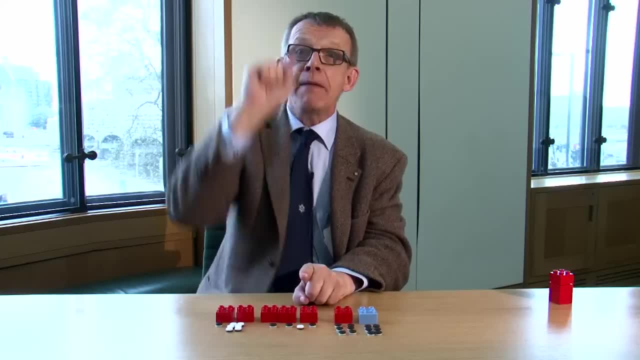 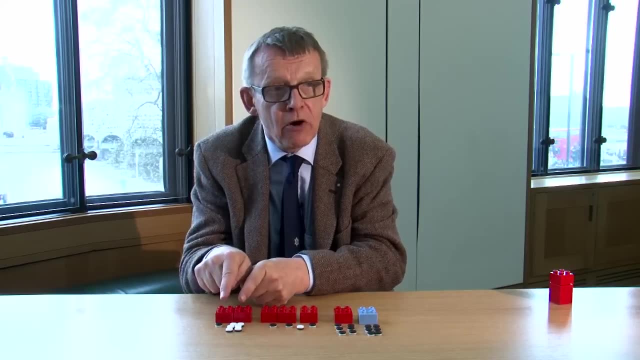 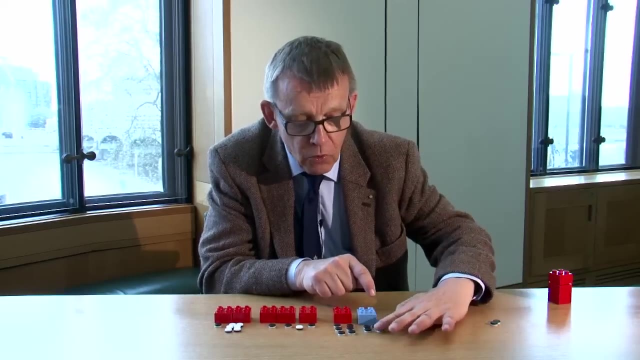 The people here in the middle. they hardly emit anything at all. They just have a lamp in their house And the poorest almost nothing. So the challenge for the world now is get away extreme poverty here and get these people to adapt and use less fossil fuel and use more green energy sources.